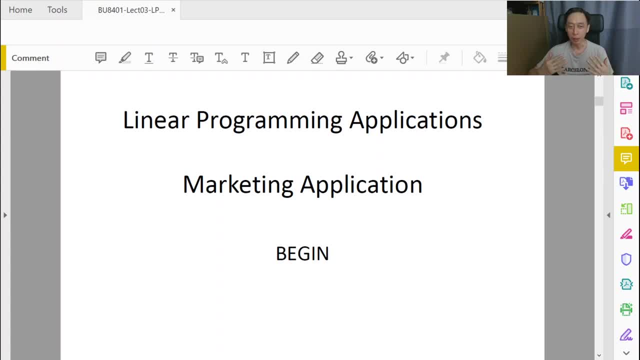 So this is Management Decision Tools, We are talking about linear programming applications and we are looking at our first example. And we'll go slow first, because this is our first serious, step-by-step manner of translating a business situation that we will present as a slide, as a description text Of 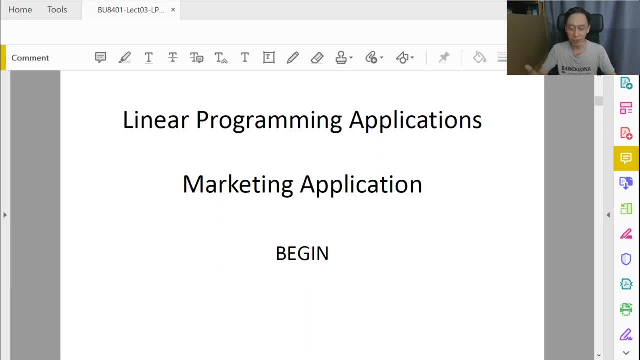 course, in real life we will have to walk the ground to appreciate the scenario. but here, given the limitations of, you know, academic learning environment, we will just present to you the business situation through a slide of text. Okay, so here we have a marketing application. We'll go slow at first and along the way. 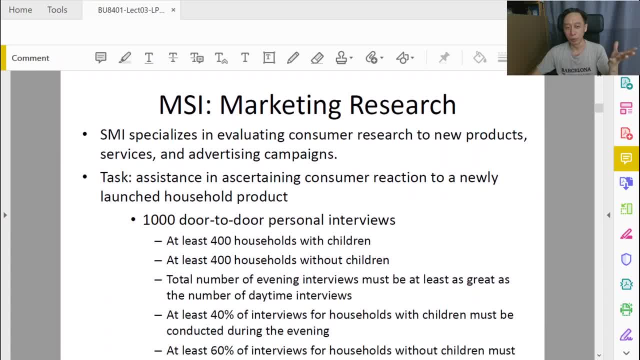 I will open source my mind to you. In other words, I will make an initial guess or initial version of my appreciation of the problem, translate it to the model, and it may not be the right version in the first case. All right, so I 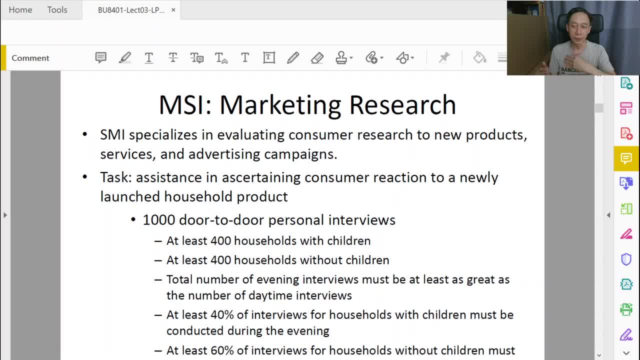 may make some incorrect version of the model along the way, and I will show you how. I discover myself that the first version is not right and I correct it so as to get the right version, And in doing so I want to show you that it is not. 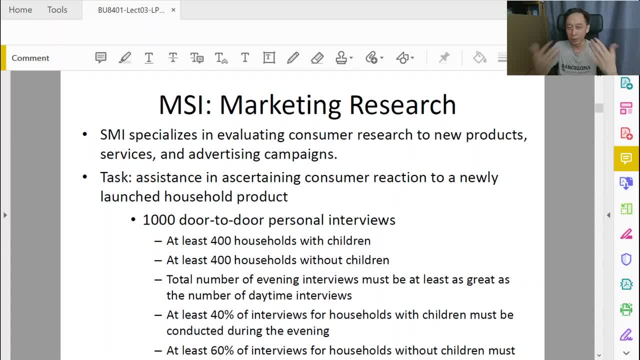 something that I have And it is not" it takes years for you to acquire. it is something that you can learn to pick up right the skills to write down an LP model that is consistent with the description in the text. so if the business text has certain constraints, 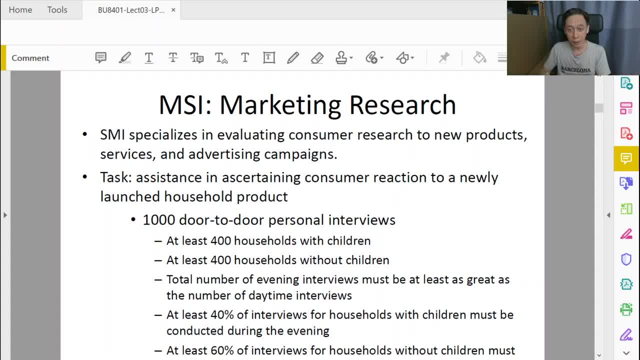 have certain concerns, you should express them in the model and I'll show you, by way of making mistakes, to how to correct your own initial, incorrect appreciation of the of the situation. all right, so we'll see how that goes now. we have a task here: to conduct marketing research enough, in other words to collect survey. 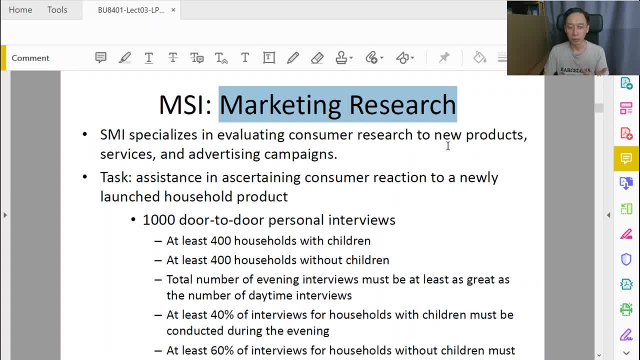 outcomes about a product. okay, so that's very common. but of course, we always have two big sets of constraints. right, we have resource limitations. whenever you hear about resource limitations, you will use less than equal to- okay, so example. what are some examples of resource limitations? budget, right, should not exceed labor hours- okay, so resources in. 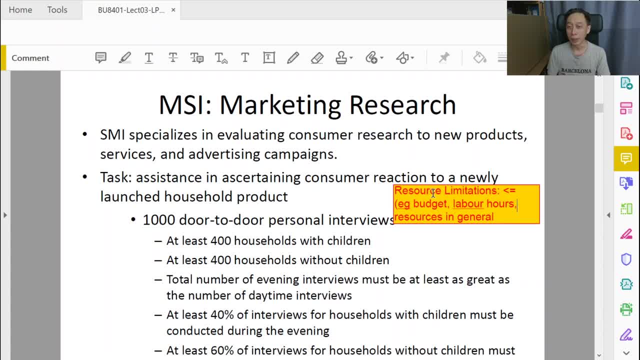 general and resources can be, hours can be, can be man count all right number of workers, resources in general. so whatever is taken as resource and in general, if there are performance requirements, that would always translate into greater, equal to. so what are some examples of performance requirements must have right. 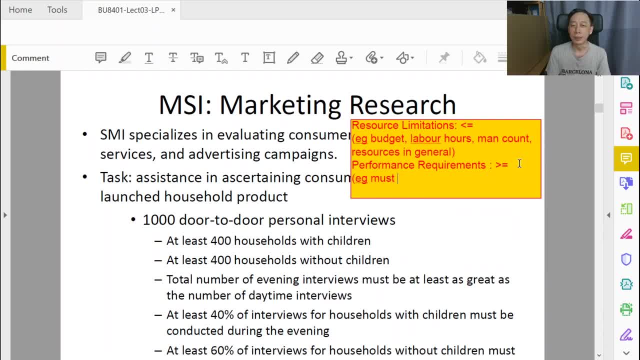 example, must produce certain outputs, must achieve certain results. make sure, on the weekly basis, we achieve $10,000 of profits. right, must do something, must attain certain expectations. okay. so, example: your GPA must be at least 2.0 to stay in the university. example: right? so these are. 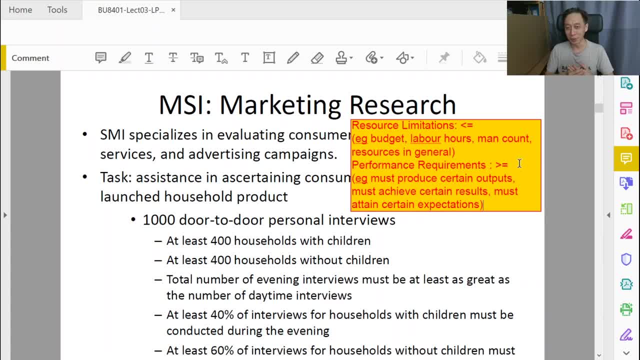 the constraints and before you take up a course you assess: will this course give me a C or D? that pulls but down my GPA and so it becomes a risky course for me, right? but if this course is kind of easy to get A plus, yeah, I think I will be. 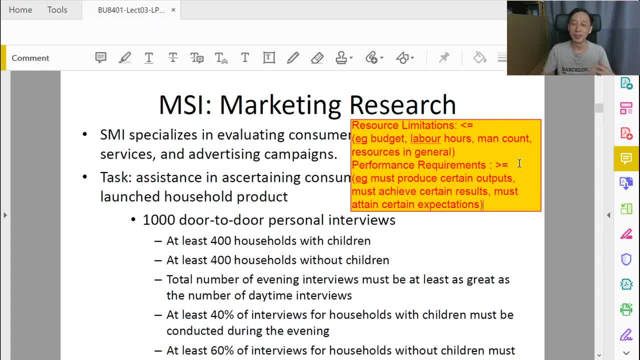 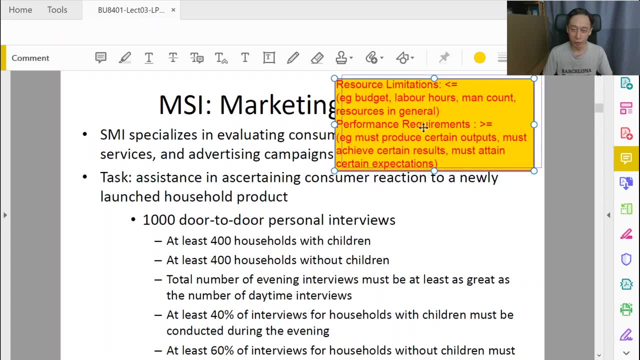 able to satisfy the university's constraint easily, so I will tend to want to do it on a greater basis or take up the course. so these are, uh, constraints that will change your behavior, your, your choice and therefore your decision. so these two groups, two big groups of constraints, are always 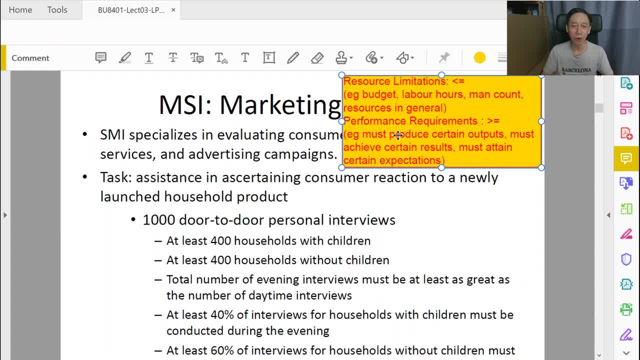 there. they are always there in almost all situations, all LP models, so definitely keep track of them all the time and because of that I will not go through too much of those two big, big categories of constraints. okay, so in this example I want to know how to define decision variables. that's one big hurdle for most. 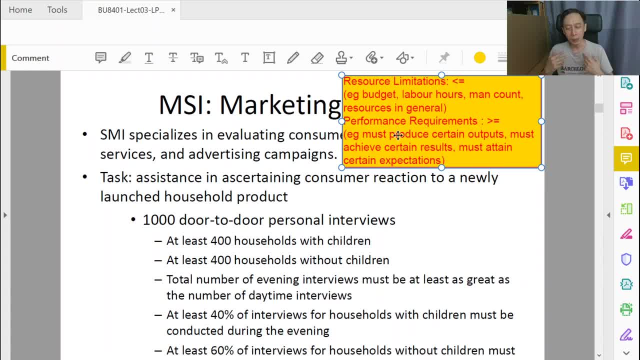 beginning learners in LP. uh, what are the decision variables? how do I identify them? anytime you have the business owner, that is the, the question asking how many, all right first, I wonder how many right. I wonder how much certain quantities have to be in order to fit in. therefore, there is no bottom line, because I know one or I. 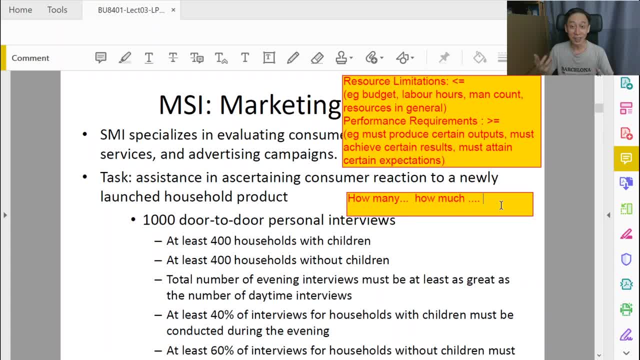 just do not matter, since, getting back to the point where you have to tell my menu exactly which one, with which demand, you have the most quantity, this time you write first question marks. um, because looking at Melanie Bob and record, for example, I wonder how much flour I should pour in, you know, so that the 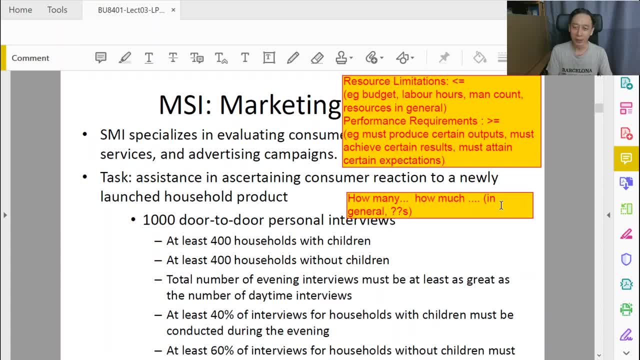 fragrance is maximized sounds like a decision variable, Then that implies that you use, you define one decision variable for each such question mark, each such quantity, All right. So this is a general guide in terms of saying: you know when a problem presents itself as 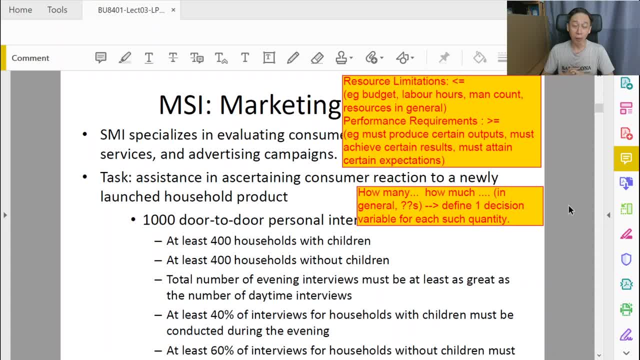 hmm, I wonder how many workers I should deploy so that the work can be done quickly. Now, of course, deploy as many as possible, right, But I only have 10, of which only two are available in the morning, another one available in the afternoon. 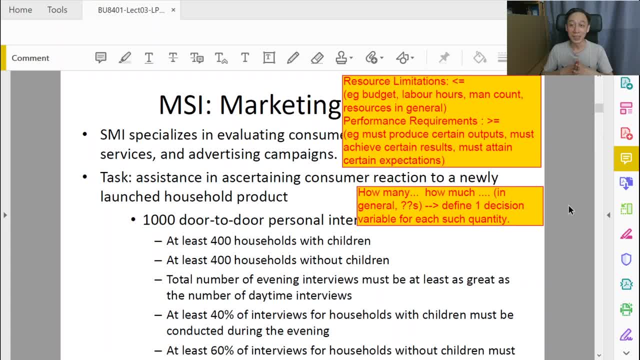 Yeah, so you start to see that, well, it's not so easy to come up with an answer even for such a situation. But that exactly means that each- I wonder how many, Each of the I wonder how much, deserves a slot, a decision. variable container right. 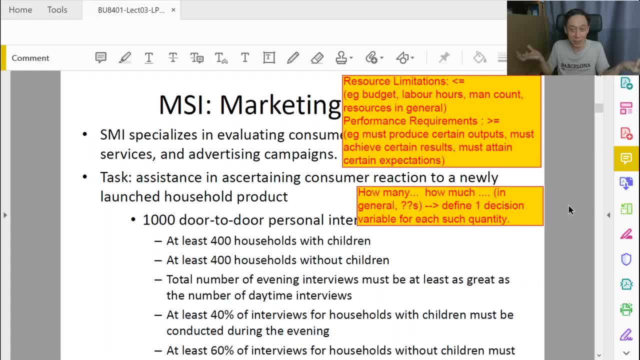 For Excel solver ultimately to deposit a number there and thereby advising us, advising the business owner, how much and how many, so as to obtain the best results. Okay, so that's again a general guide: how much, how many. So let's apply them. 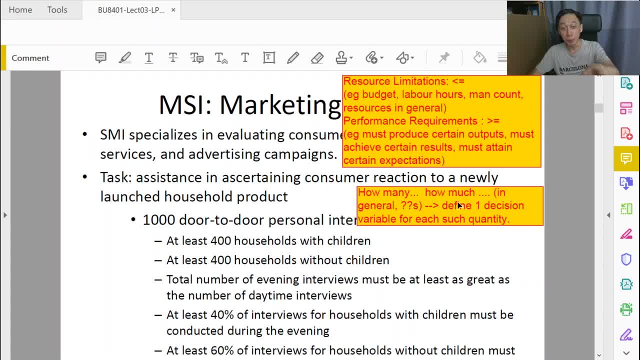 And try to come up with a, with an LP model to describe fully this marketing survey project. So everything is quite straightforward. It says we require all these constraints to be fulfilled. What are they? We need 1000 door to door personal interviews. 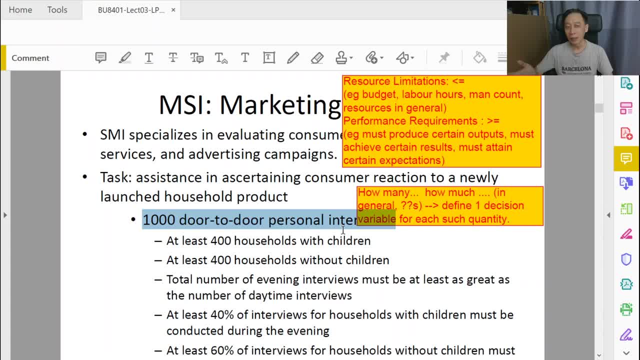 Fine, If that is the only constraint. give me the money and I will implement and hire enough people to knock on doors to get you 1000 outcomes, because there's no room to negotiate, There's no room to optimize. 1000 means 1000, right. 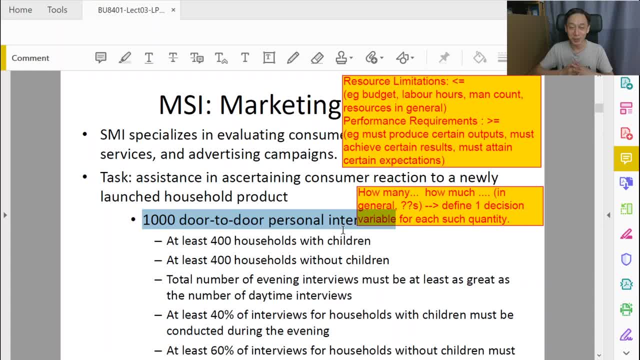 You cannot say: let me try 900 because that doesn't satisfy the constraints. so that cannot be it. But I do imagine, as I read right, it will be the case of something like saying that I will have a decision, have a constraint, that on the right hand side it is 1000.. 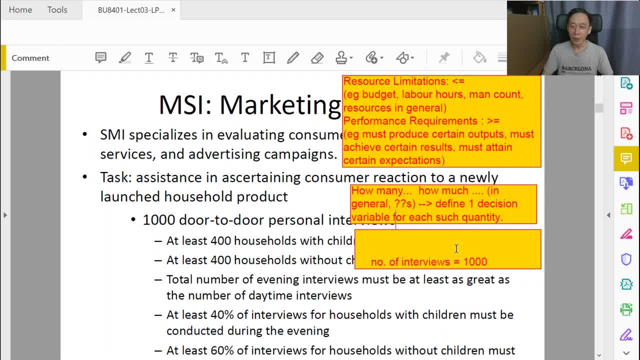 So I'm kind of like: number of interviews, right. So this constraint will have to be in, except I don't know yet how to describe number of interviews. That could be one variable, n, right, Let n be the number of interviews subject to the constraints. that n equals to 1000, finish. 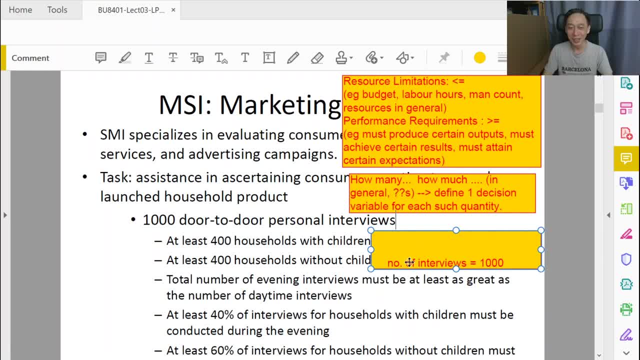 But of course it's not very interesting, right, Because you can solve it right away. Okay, But let's move on and see at least 400 households with children. Oh wait, Okay, At first I only have one decision, variable n, right. 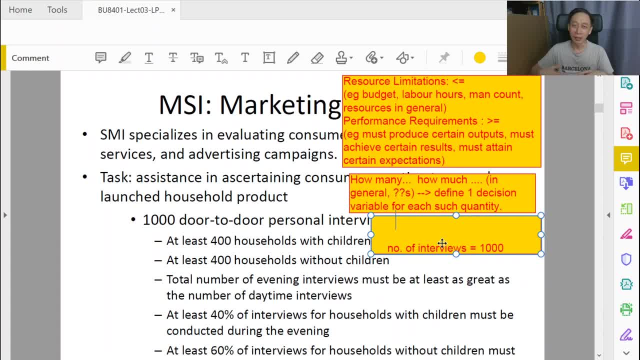 And I constrained n to be 1000. So n cannot be 999,, cannot be 1000.. Fine, But now I have no way to describe households, that is, children, interviews with children, households with children, I cannot describe. 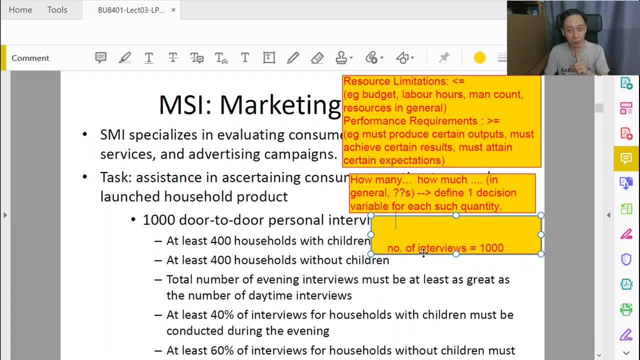 I can only describe that if I only have one decision variable, because that decision variable is always having the value 1000. So I wouldn't be able to say something like at least 400 households, that is, interviews must be done with children, households with children. 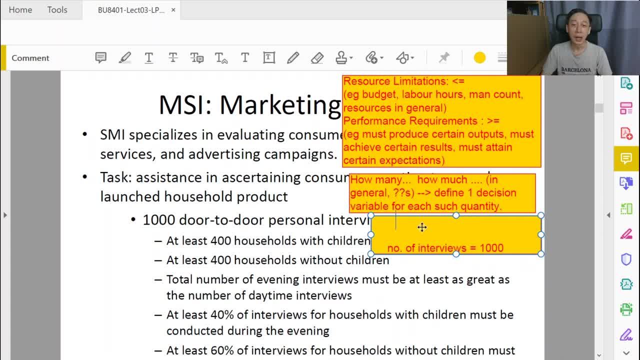 So well, instead of one decision variable, I now have to split. let me move it on the left hand side. I now have to have two decision variables, right? So I need to say that instead of saying n, right. 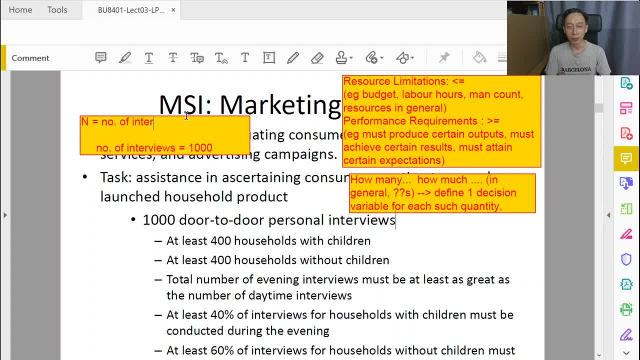 Equal to number of interviews. I cannot do that because it's not enough bandwidth for me to describe two numbers- households with children, households without children- So I have to write it as no children interviews done on households without, with no children and children right. 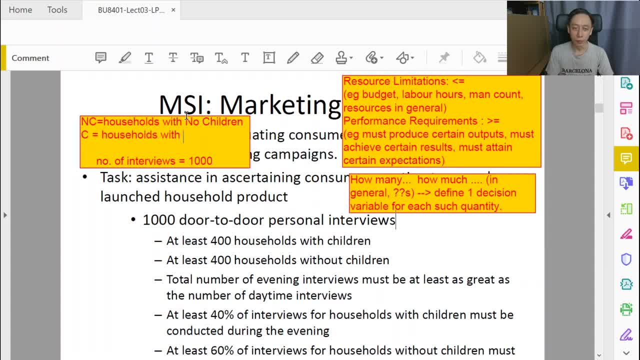 So Okay. so now I have two variables and I know that they must add up to 1000, so now I need to change this into nc plus c see that? So I haven't invalidated any of the previous constraints, but now I have more bandwidth to entertain these constraints, and I can say that with children, right? Households with children Has to be at least 400, and the second one, households without children, also has to be at least 400, leaving the room for c to be 400 to maybe 600, and nc could also be 400 to 600.. 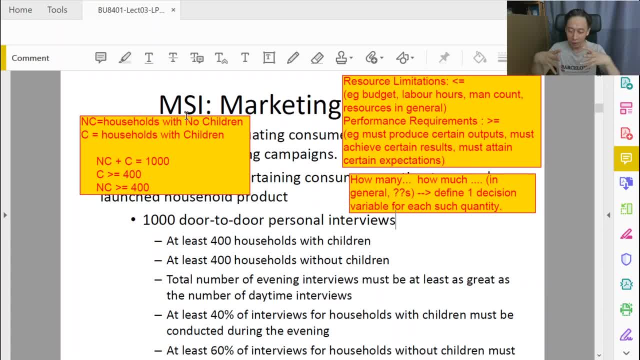 So there's a rubber band range now and in this space we will have to optimize it right by minimizing the cost. So so far, so good. I'm up to the third constraint. Total number of evening interviews must be at least as great as the number of daytime interviews. 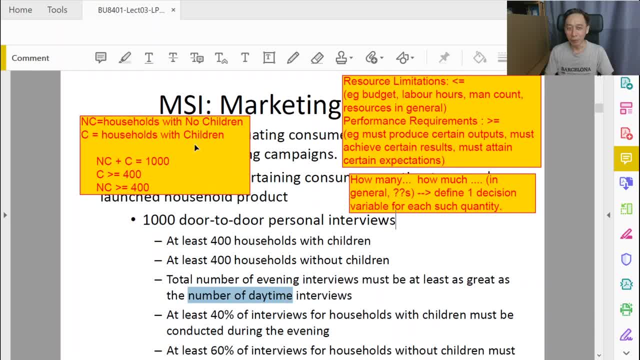 Okay, So, as you see, now we went from one total to children without children, and now we have this additional, rather orthogonal kind of description called daytime and evening time, Right, So? so it is about two kinds of time slots, and both households- with children and without children- can be done in the daytime, can be done in the evening time, giving us a two-by-two matrix. Right.